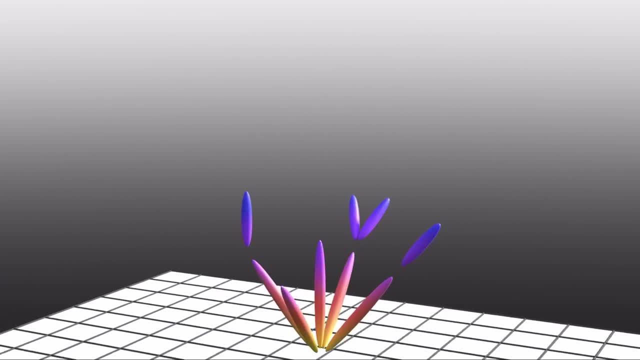 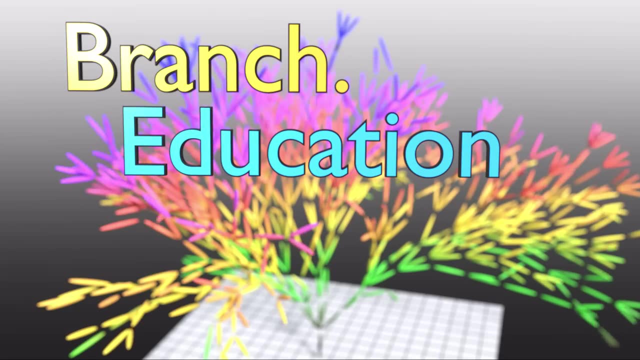 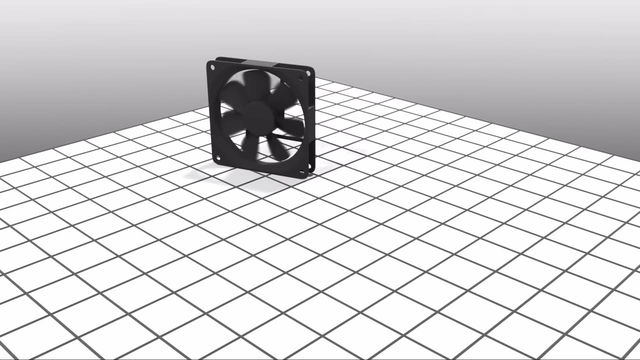 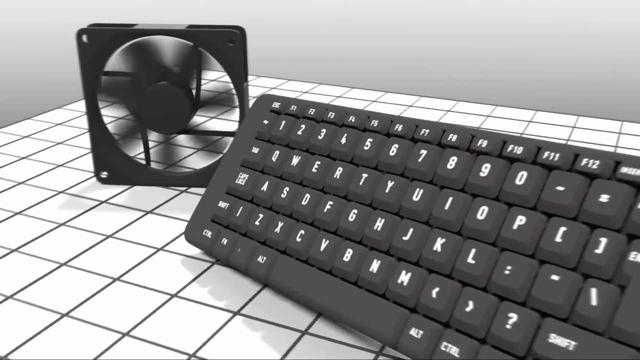 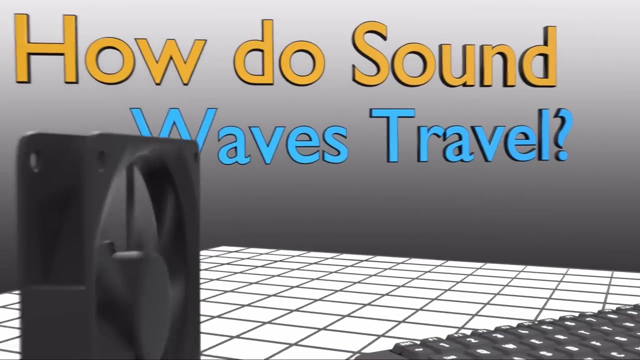 Every waking second of our lives, we hear sound waves everywhere, From the hum of a fan to the clicking of your keyboard. sound waves permeate our lives, But how do they travel throughout the world around us? To answer this question, we are going to engage in a thought experiment. 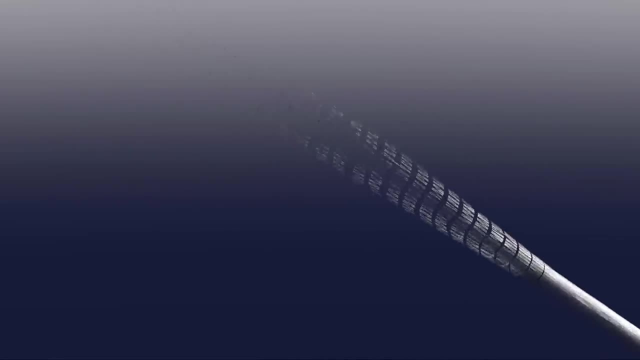 Okay, so let's say we have a bar of steel that reaches the 384,000 kilometer distance between the surface of the earth and the surface of the moon overhead. Let's be real, that's a very long bar that could never feasibly exist. But for the sake of this thought experiment, let's say it. 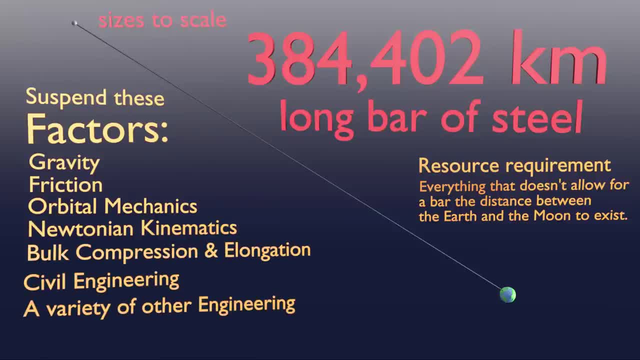 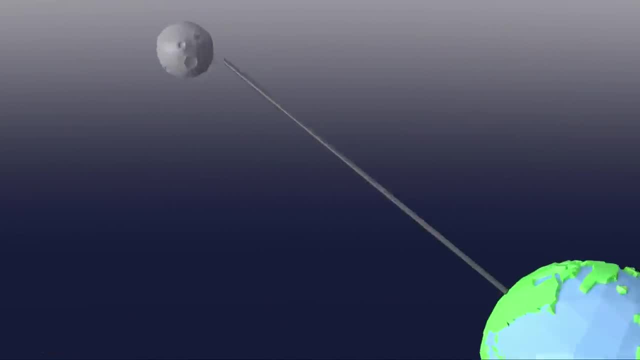 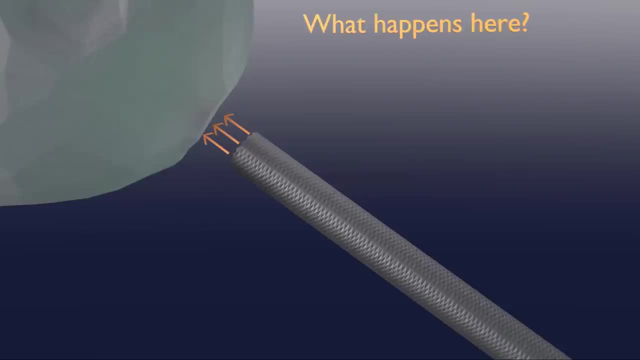 does and that we are going to suspend all of these factors. Let's pose this question: If we were to raise the earth side of the bar by one meter, what would happen to the far moon end of the bar? Would it move a meter instantly? Would there be a couple seconds delay, Possibly an hour delay, Or maybe? 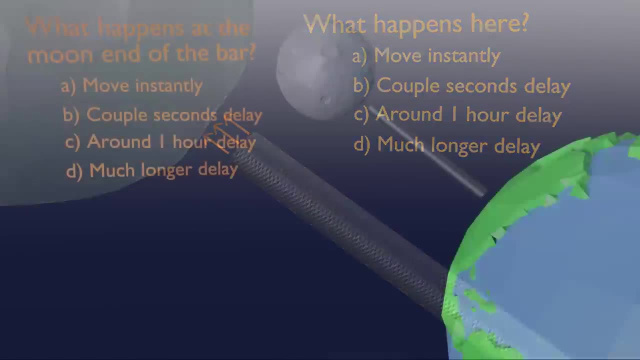 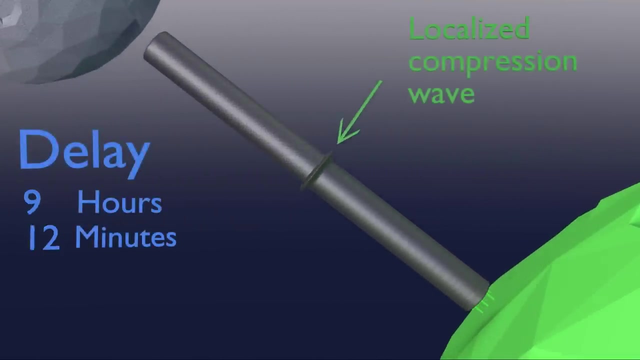 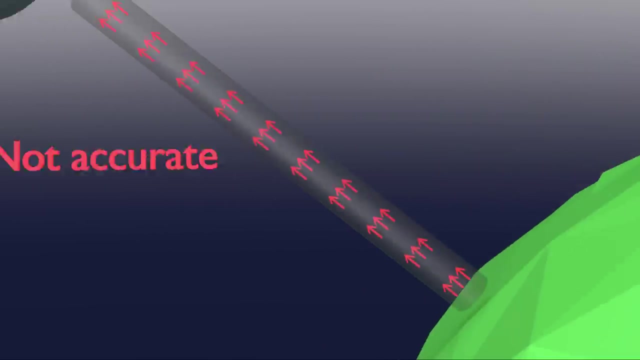 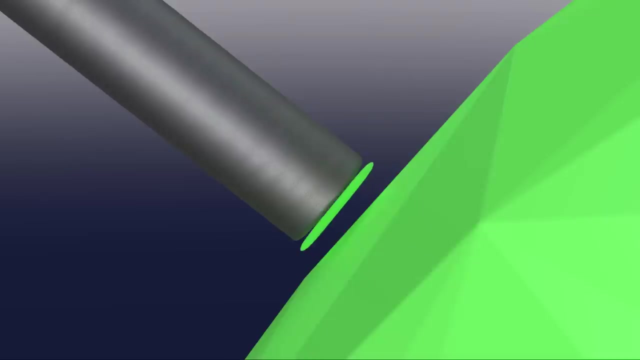 much longer delay. As it turns out, the moon end of the bar would move one meter 18 hours and 24 minutes after we moved to the earth end of the bar. This is a massive delay, And it is due to the fact that when we push on the bar on earth, we are not pushing on the entire 384,000 kilometer long bar at once, but rather we are just pushing on this localized group of atoms here. 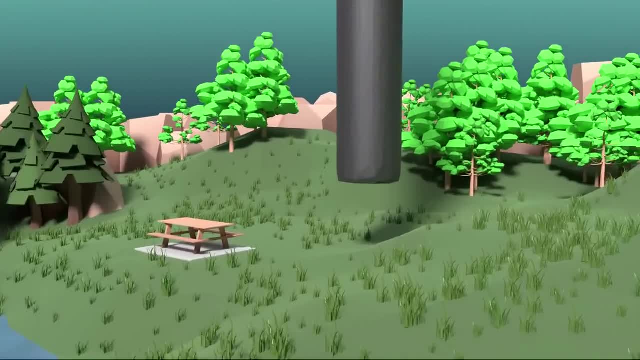 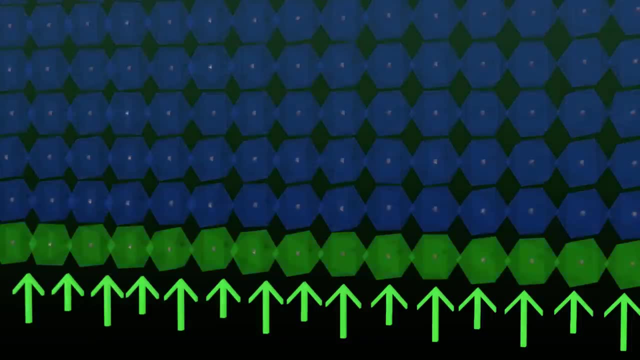 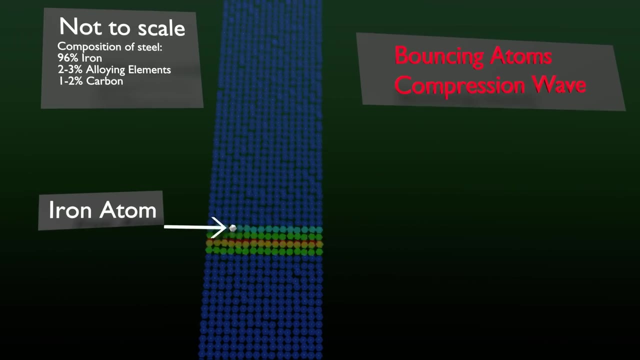 How far is it in times ofvasive attributed to that, daar Pv Qy. These atoms at the earth end of the bar push on their adjacent atoms, and then the next group of atoms up the bar, and so on all the way until this pushing reaches the moon. 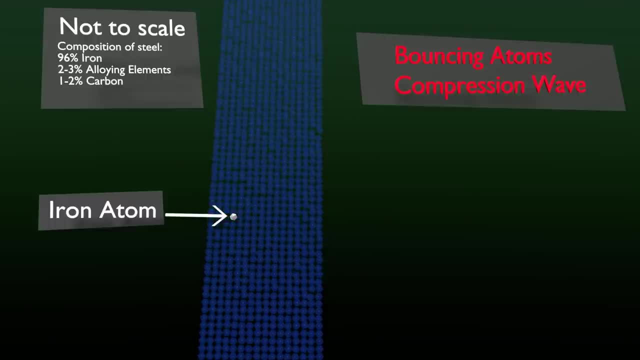 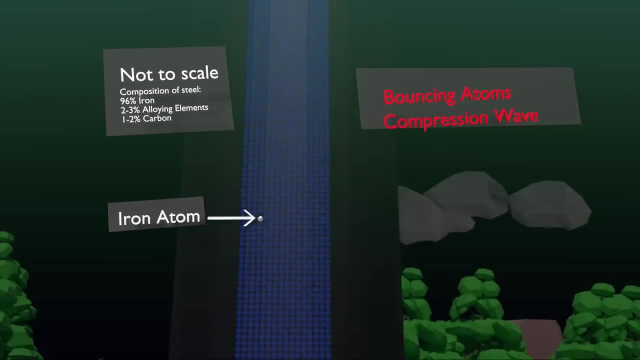 So this pushing can also be thought as a bouncing of atoms, and it does not travel up the bar instantaneously, but rather it takes time for one VarIq nastoyteצki group of atoms to push or bounce into the next group of atoms. 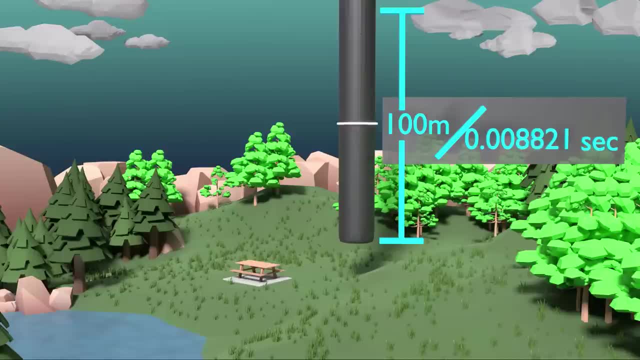 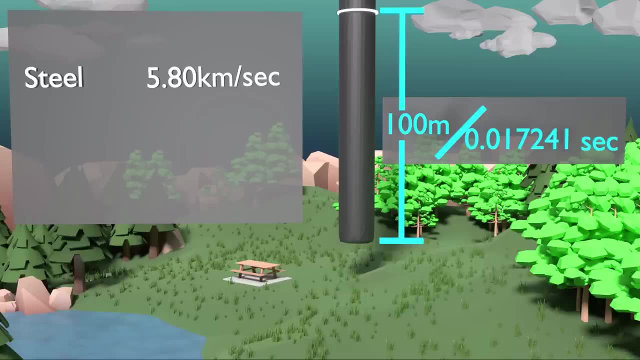 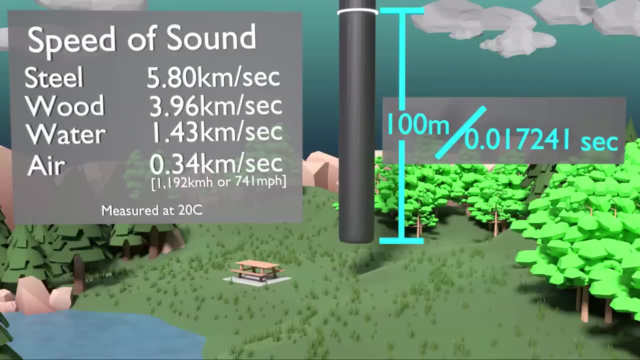 Specifically in steel. this rate of bouncing and reacting to the adjacent atoms travels up the bar at a rate of 5.8 kilometers per second. This speed is considered the speed of sound in steel and it varies depending on the material. If the bar were made of oak, the distance between the earth and the moon would be covered. 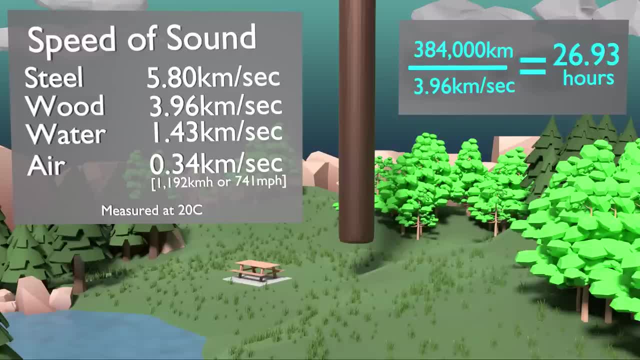 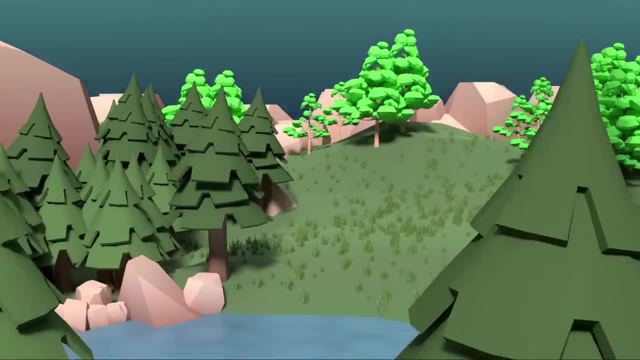 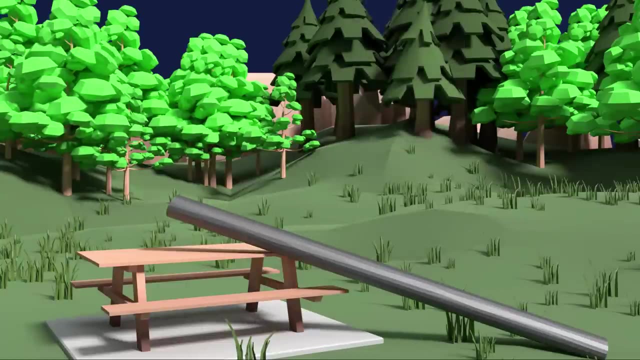 in just under 27 hours. That's a long time, but eventually the motion would get there. The point is that, although materials like a steel bar or wooden table look to be a coherent, single object, and thus one would expect the entirety of the object to move instantly, all 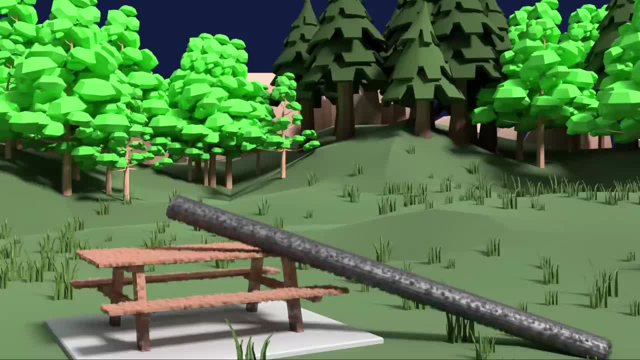 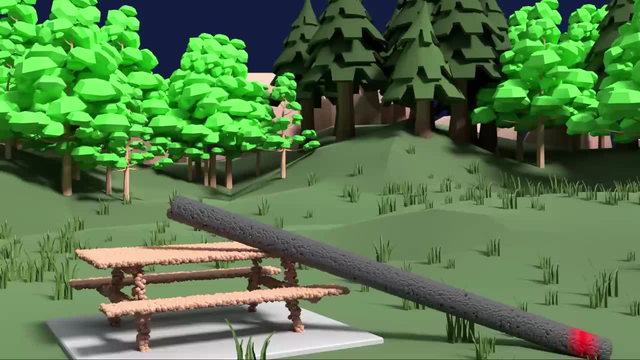 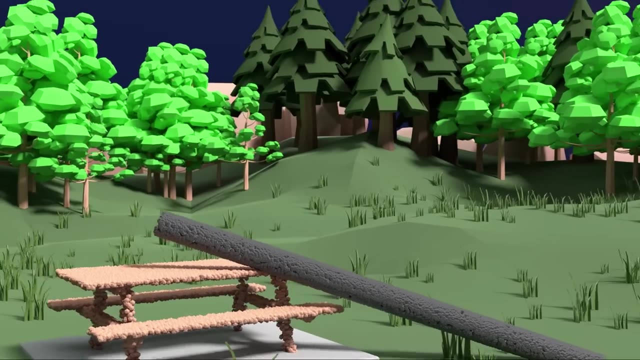 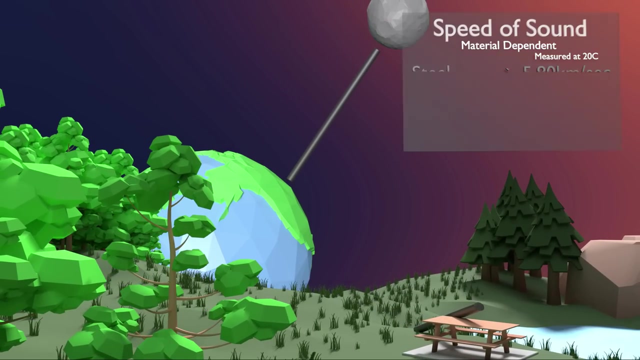 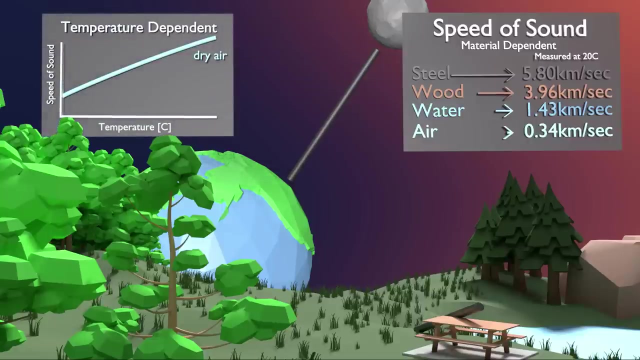 at once. In reality, forces and movements take time to travel throughout the many atoms in an object. This traveling of movement or propagation can be thought of as a chain reaction of atoms pushing or bouncing into one another. The speed of this propagation is called the speed of sound and it is dependent on the 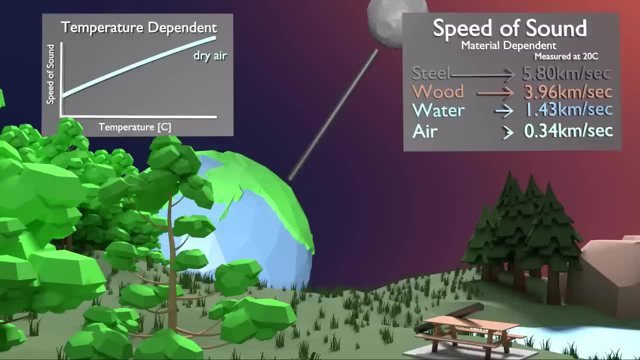 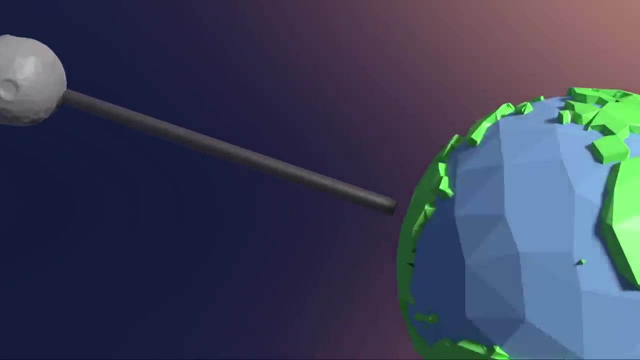 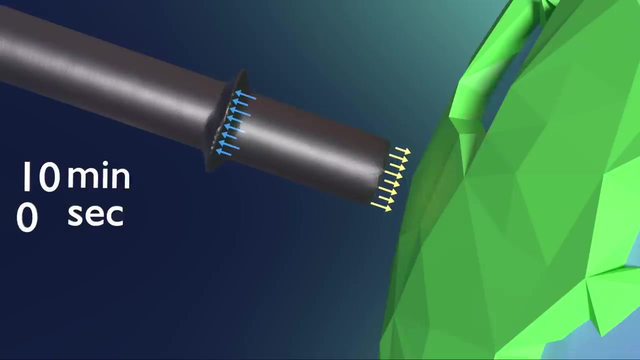 material or medium that the motion passes through. It is also dependent on the temperature of that particular medium. Now let's get back to the thought experiment. Consider what will happen if we move the steel bar differently On earth. let's move the bar up and then, after 10 minutes, we move the bar back down. 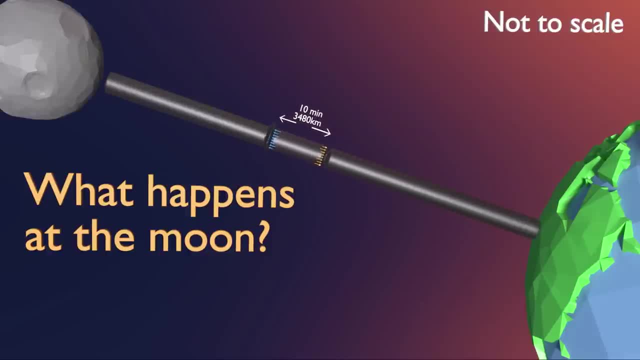 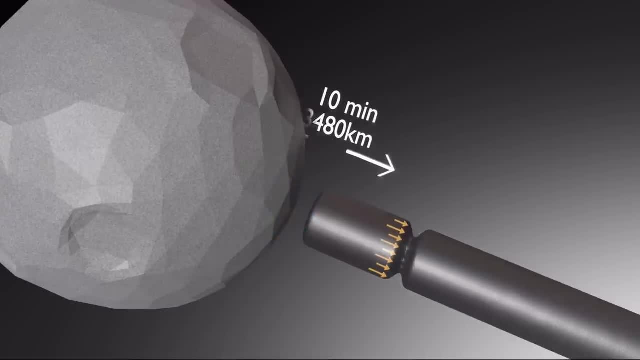 What will happen on the Moon? What will happen here? No, No, as much. N MCU: No. This is exactly what happened in the end. Well, similar to our previous experiment, after 18 hours, the bar will move up and then 10. 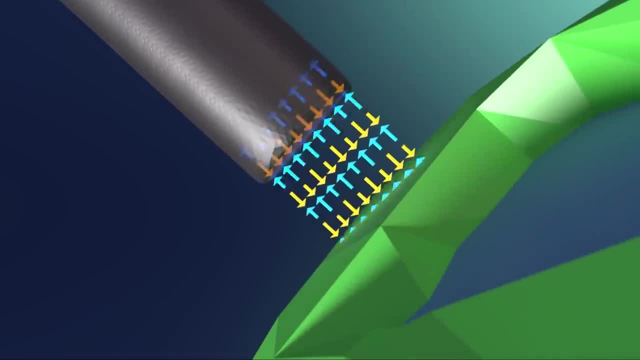 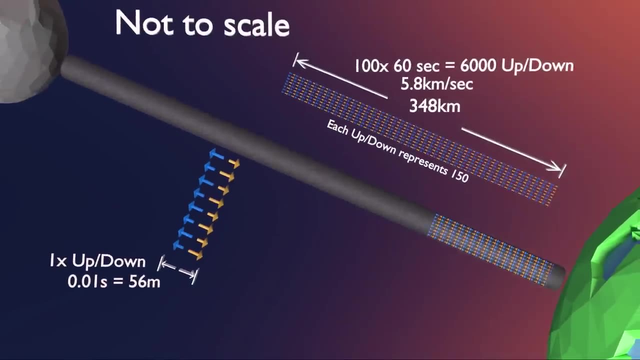 minutes. after that it will move down. Now let's say we move the bar faster, specifically up and down 100 times a second for a full minute, and then stop. Well again, this shaking like motion will start at the earth end of the bar. 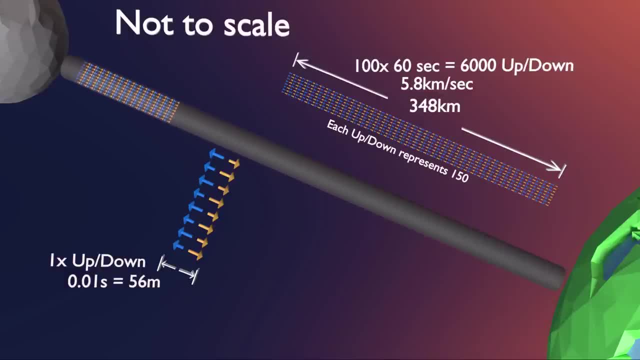 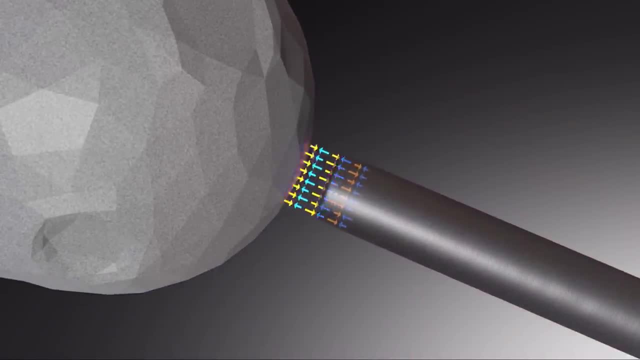 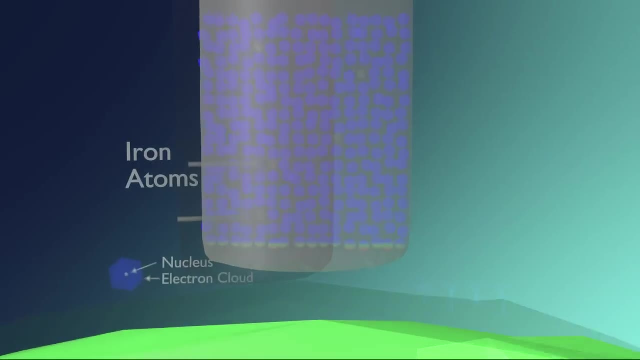 make its way up the bar at a rate of 5.8 kilometers per second, and after the 18 hour delay, the moon end of the bar will move in the exact same shaking motion for one minute. in essence, forces and motions in a material do not catch up to one another, even if the forces. 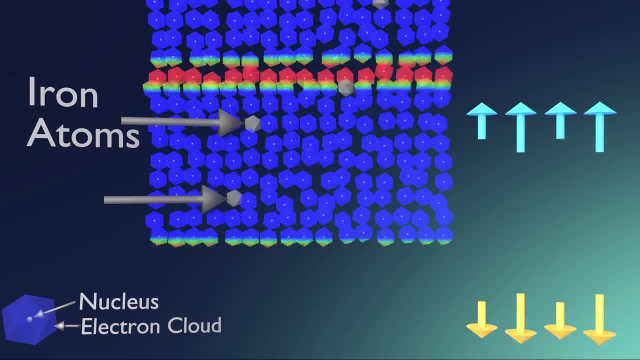 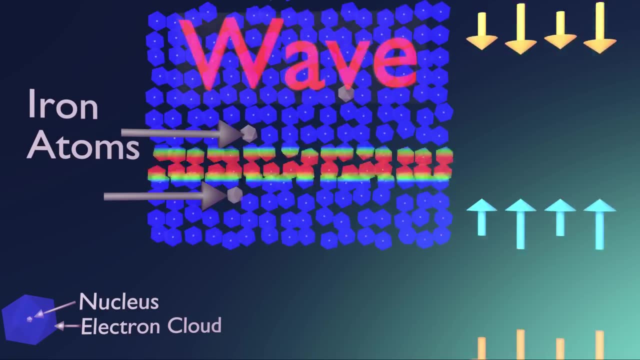 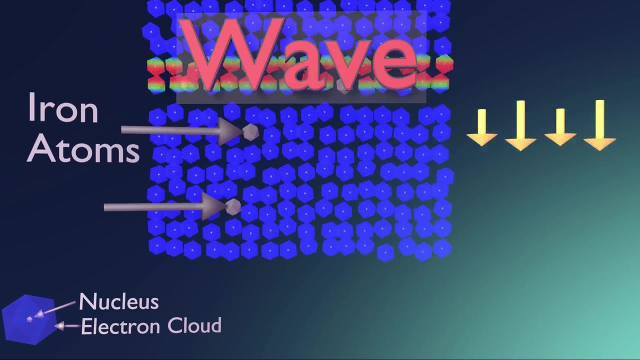 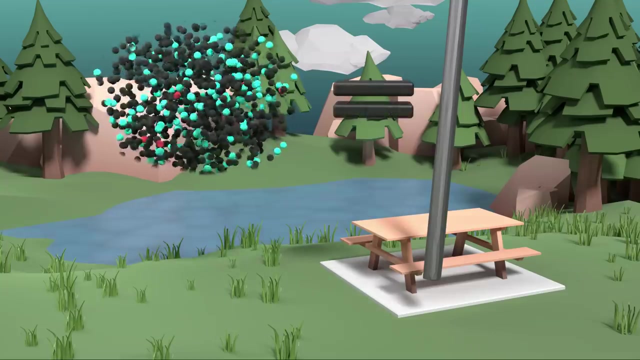 are in the opposite direction, but rather, once a motion is started, it continues up the bar at a constant speed. the propagation of this motion is called a wave. in this thought experiment, the steel bar represents the air around us in the chain reaction of bouncing atoms up, the steel bar represents the propagation of a sound wave. 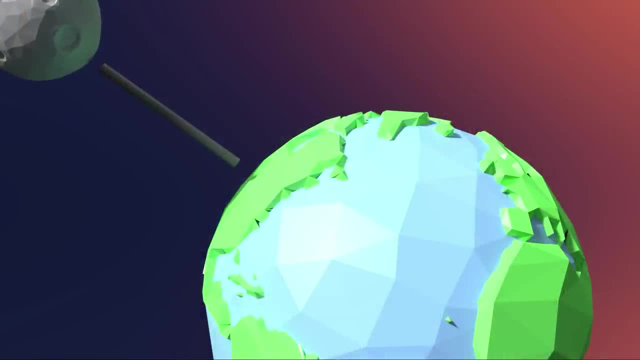 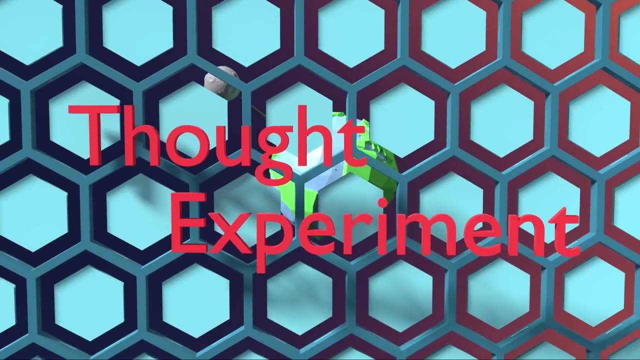 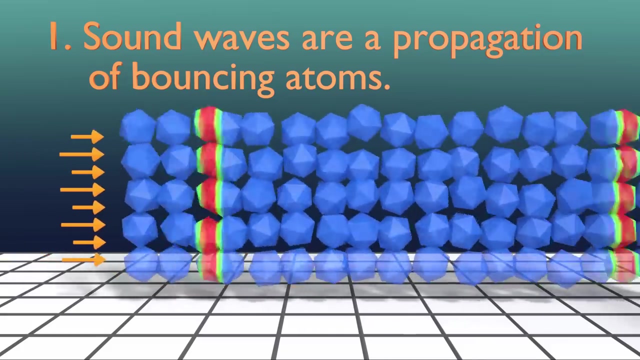 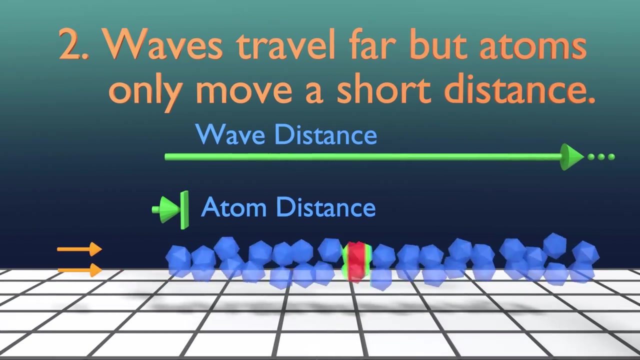 there are five key concepts shown in this thought experiment that will help you better understand sound waves and waves in general. the first is that sound waves are a bouncing of atoms or particles into one another. second, waves can travel very far. however, the atoms themselves only travel a short distance. 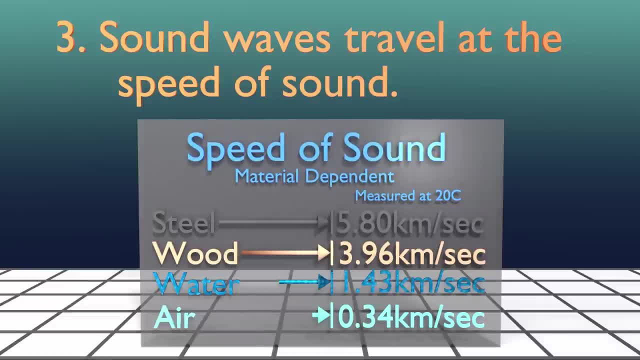 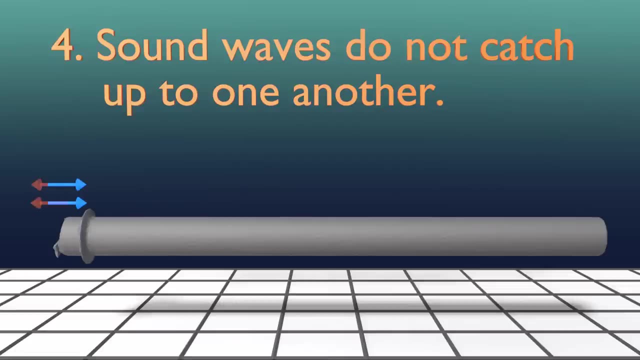 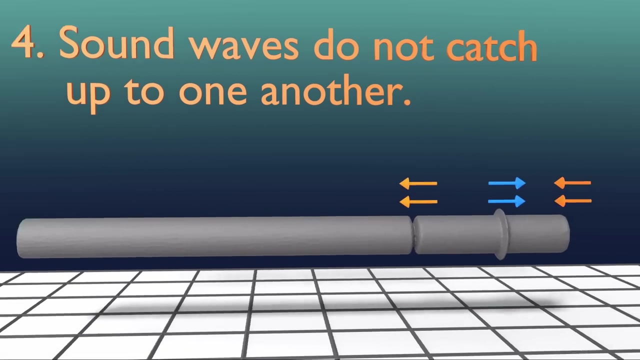 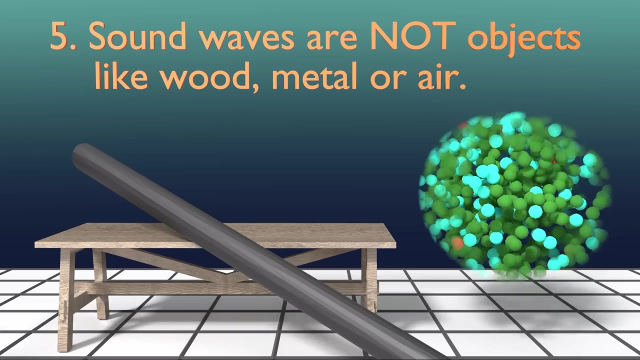 third: waves travel at the speed of sound, and these speeds are material dependent. fourth, sequential waves in the same medium travel at the same speed, and thus one wave does not catch up with the following wave. and finally, fifth, the coup de grace of consciousness: a sound wave isn't really an object like a steel bar, a wooden table or atoms of air, but rather 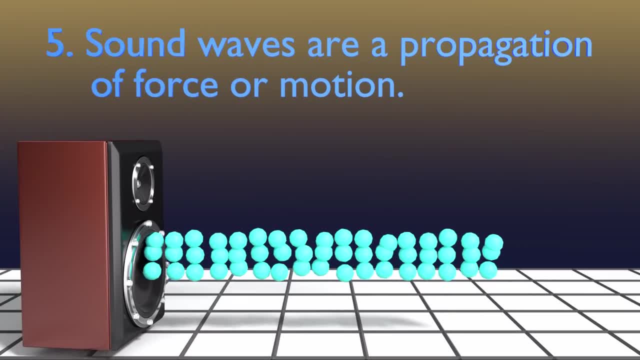 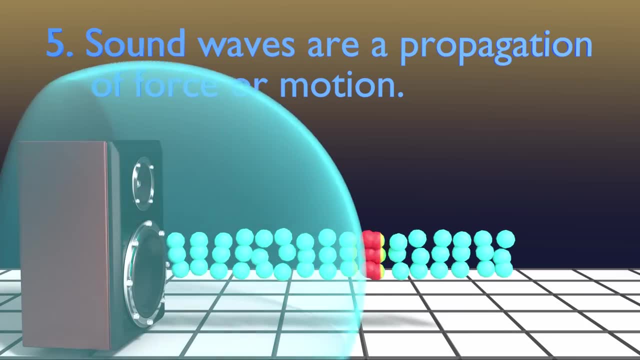 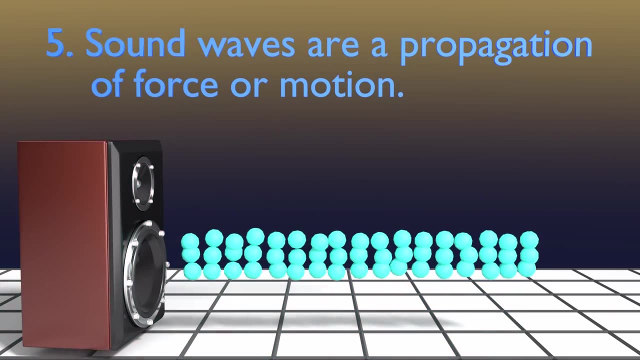 a sound wave is a propagation of force or motion. when we hear something, we are in essence hearing the motion that an object makes, or how kind of that object is applying a force to the air particles around it, thereby causing those air particles to bounce around, and that bouncing is picked up by your ears and perceived as sound kind of fascinating.